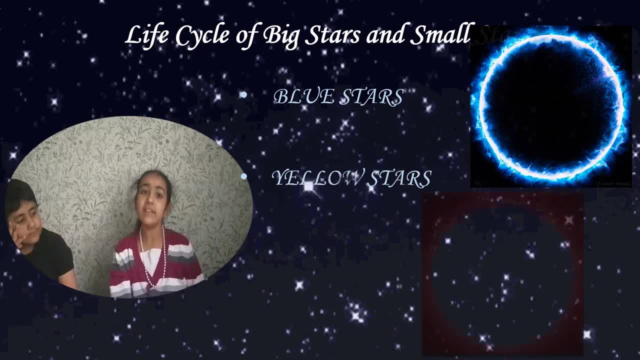 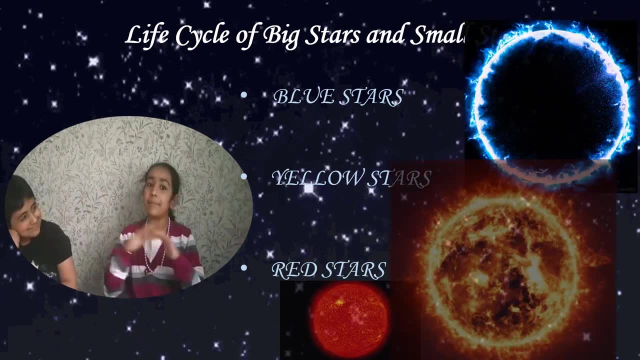 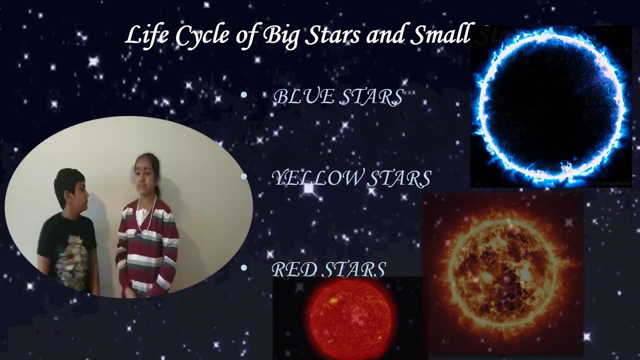 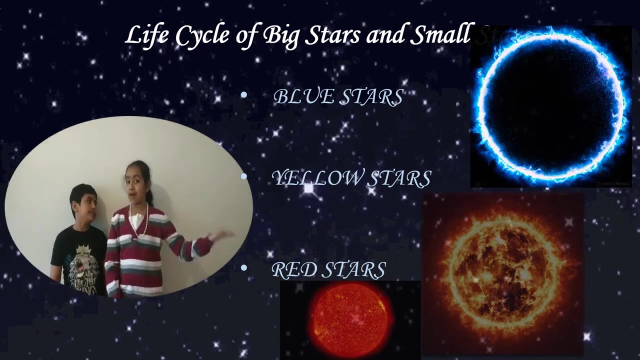 Blue star, yellow star and red star. Blue stars are big, hot and bright. Yellow stars are medium sized. Red stars are small, cool and dim. Rudraj, actually, these stars are categorized depending on their mass and temperature. Stars are small, cool and dim. 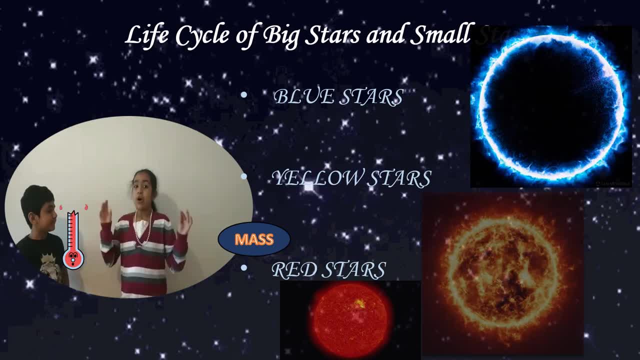 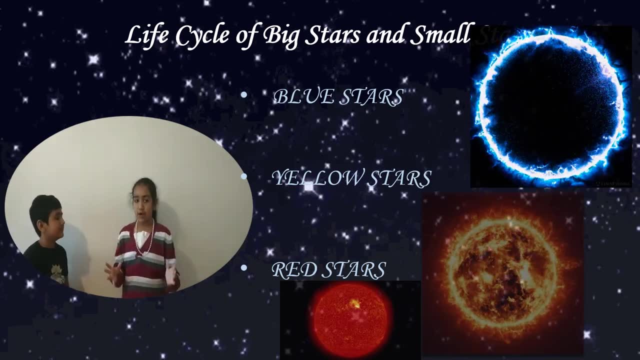 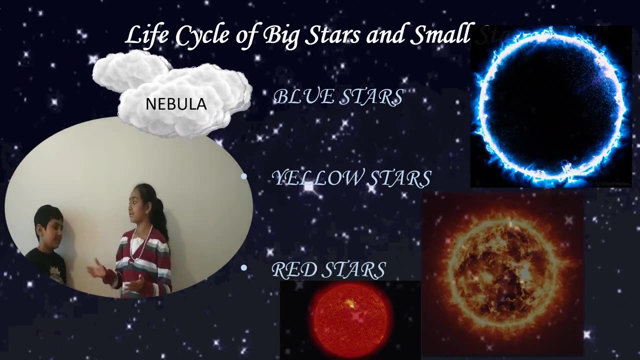 Rudraj. actually, these stars are categorized depending on their mass and temperature. These are super heated bodies of mass and they are formed from the clouds of gas and dust called stellinebula, Stellinebula Stellinebula. 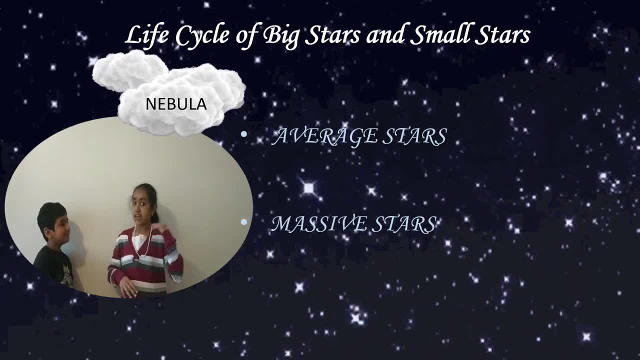 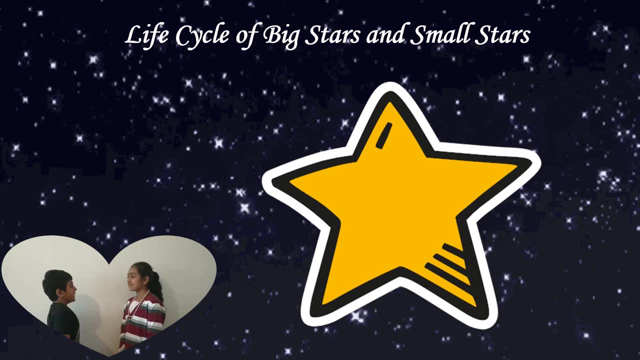 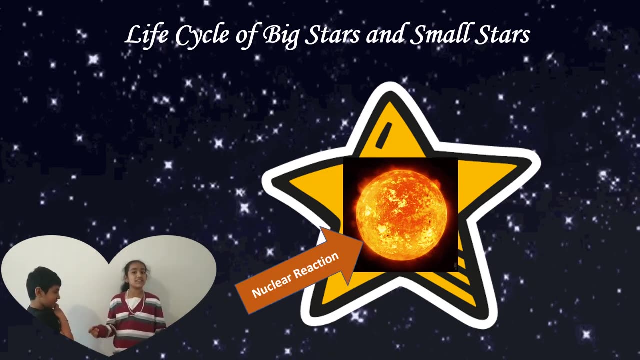 Yes, We have two types of stars: Everglades star and massive stars. How stars shine? Stars shine due to the nuclear reaction which happens in the center of the star. Okay Rudram, Okay Raina. It produces enough energy to make the stars shine brightly for many years. 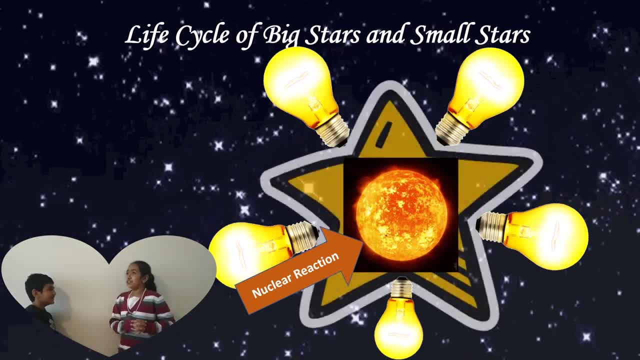 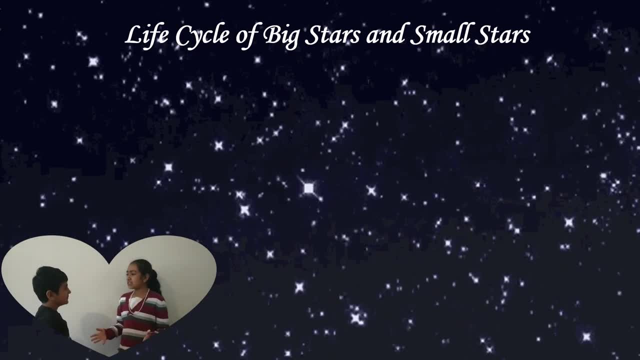 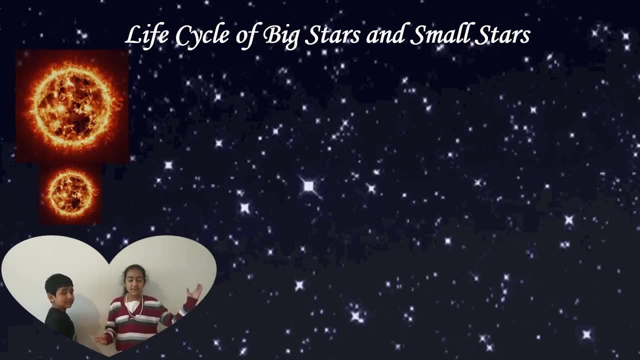 Okay, Okay, Raina Rudram, do you know how we can calculate the lifetime of a star? No Didi, It depends on its size. I will explain you how. The bigger the size of the star will burn its fuel faster. 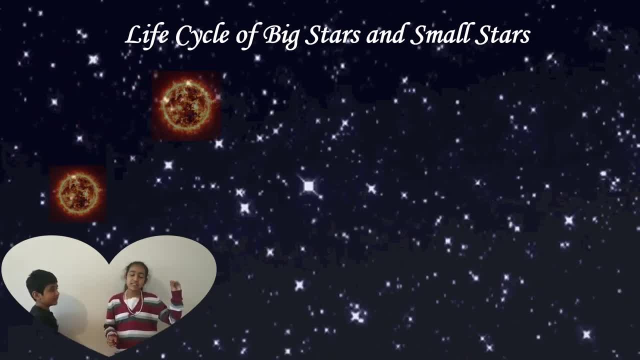 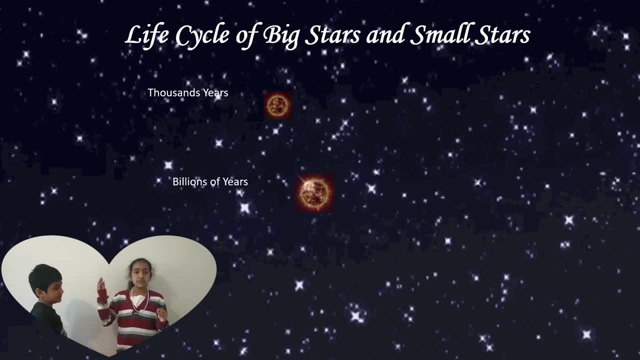 So it lasts for only few thousand years. But the smaller the size of the star will burn its fuel very fast And the smaller the size of the star will burn its fuel very slowly. So it will last for billions and billions of years. 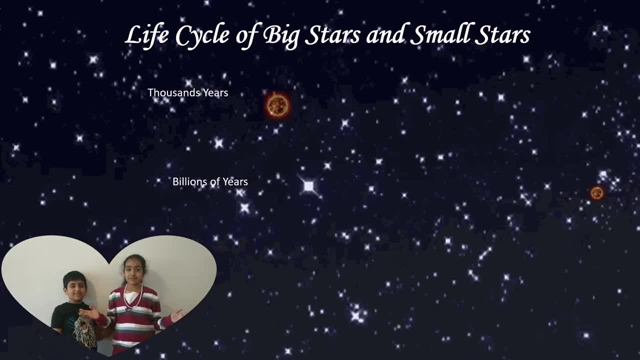 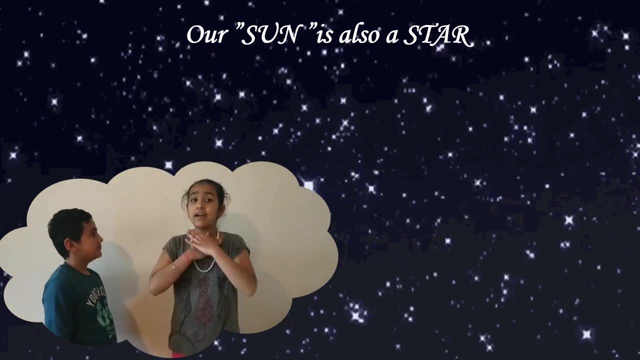 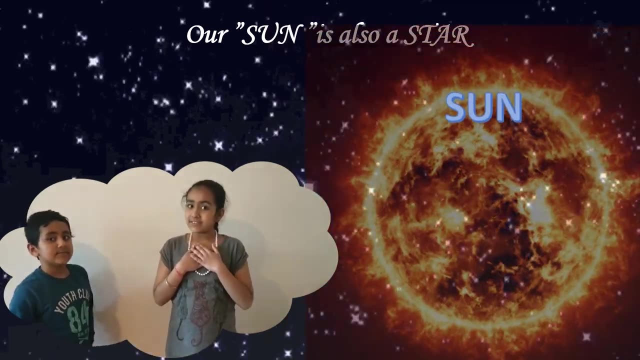 Okay Okay, Rudram. now coming back to your question, our sun is also a star. It is an average star- Okay Okay, Raina Didi- But without its energy we would not exist, And it is made up of hydrogen and helium. 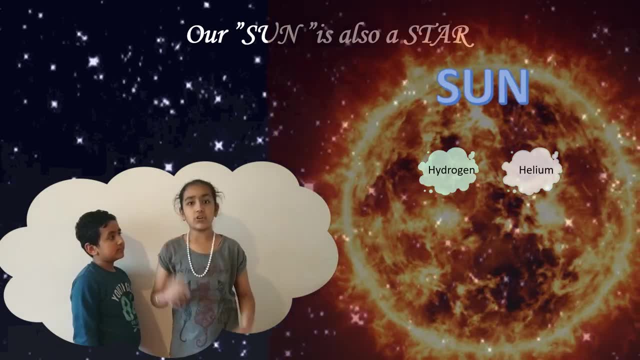 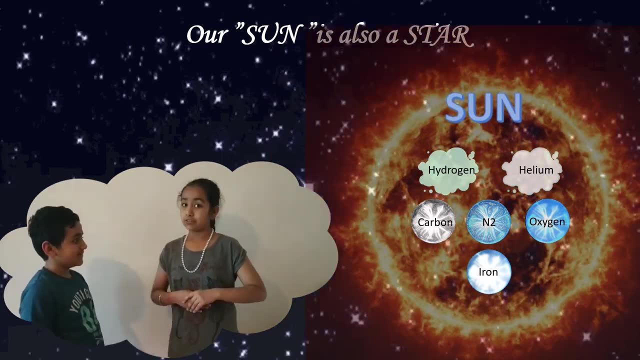 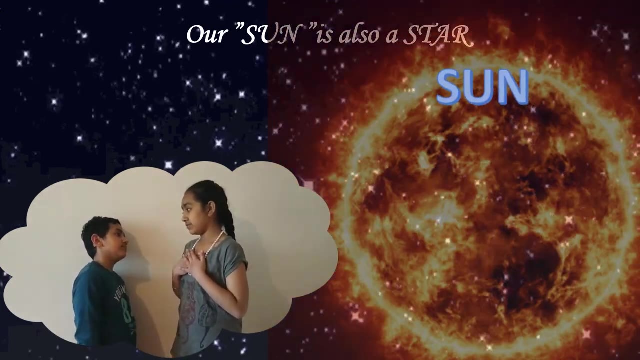 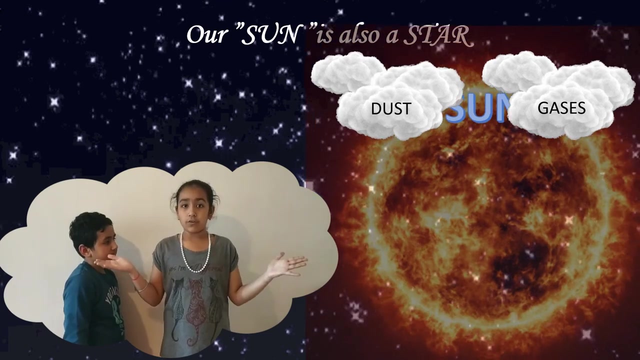 Okay, Raina Didi. Okay, Raina Didi. And little amount of oxygen, neon, carbon and iron. Okay, Rudram, do you know when sun began producing its own light, heat and energy? No, I will explain you. when dust and gas in a giant cloud collapsed under the force of its own gravity. 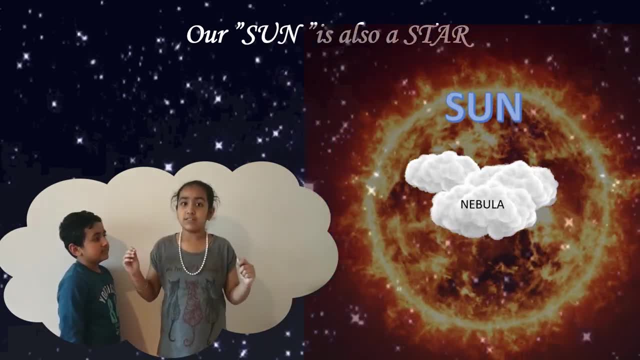 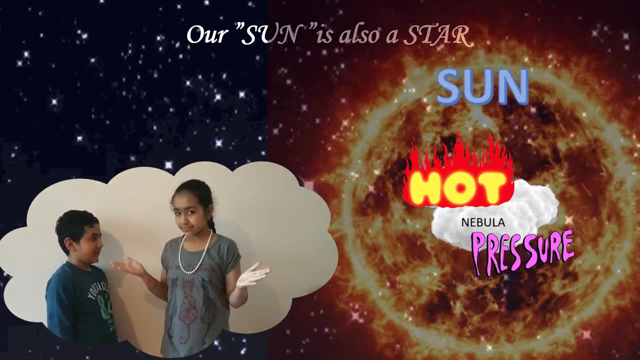 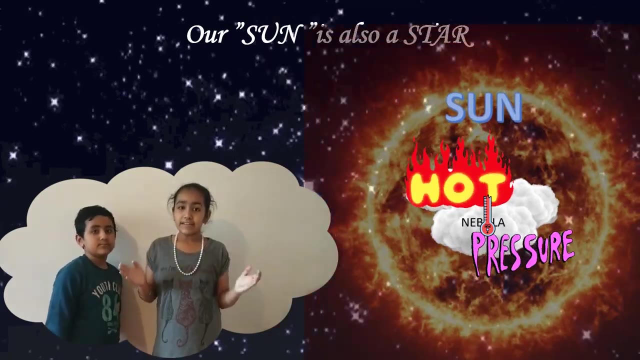 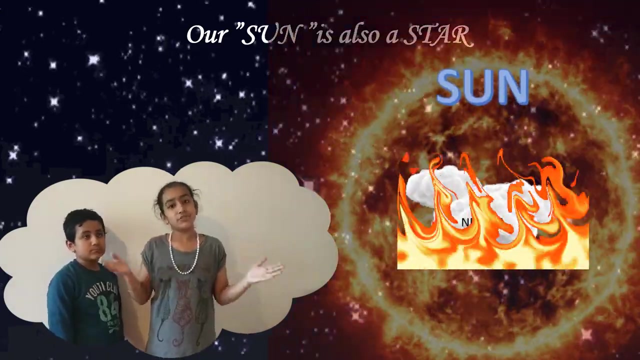 And these materials fell into the sun, And these materials fell inwards and it created a lot of heat and pressure, Okay, Okay, And when the temperature increased in the sun's core, it ignited, causing it to begin nuclear fusion. And when this happens, the sun began producing its own light. 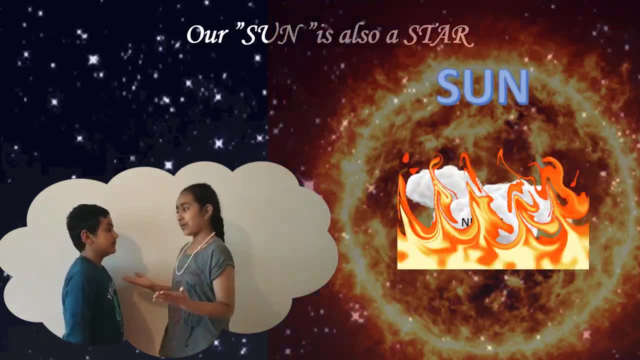 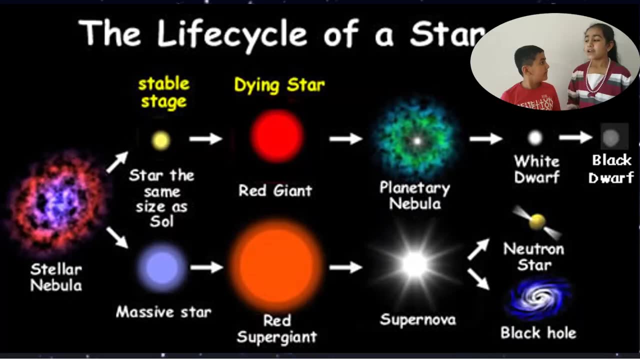 its own light, heat and energy. I hope you understand Rudraanch and you all guys. Yeah, Rudraanch, now I will explain you life cycle of star. As I have told you that life time of a star depends very much on its size and when the hydrogen fuel in the centre of 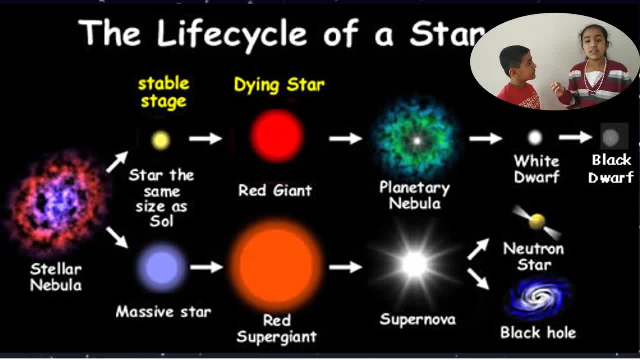 the star is exhausted, then nuclear reactions will start move outwards into its atmosphere. Okay, Okay. As a result, the outside of the star will start expand and cool. Over the time it will become red joint. Red joint is 400 times bigger than its original size. Red. 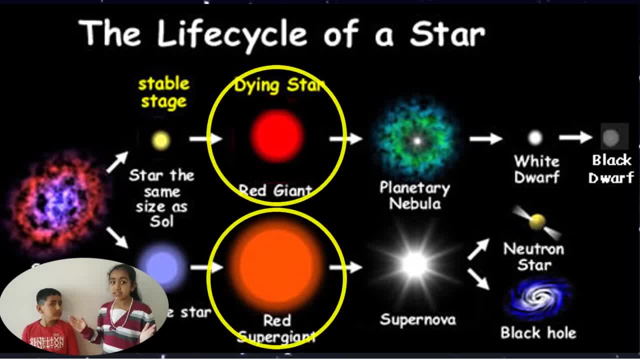 joint is 400 times bigger than its original size. Red joint is 400 times bigger than its original size. Rudraanch, can you see? here we have two different evolutionary parts: Loma stars and Pima stars. Okay, For Loma stars, when the helium has fused into carbon.